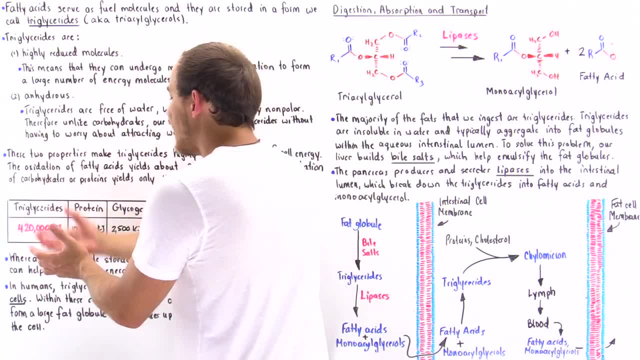 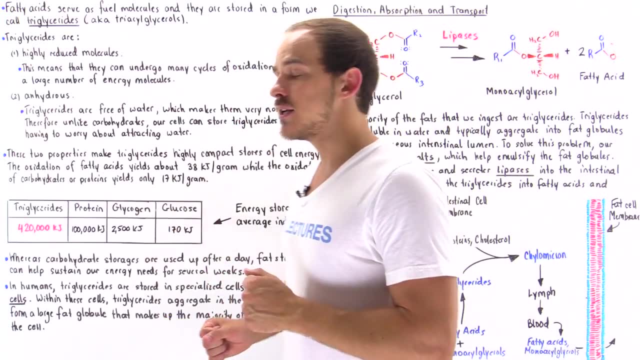 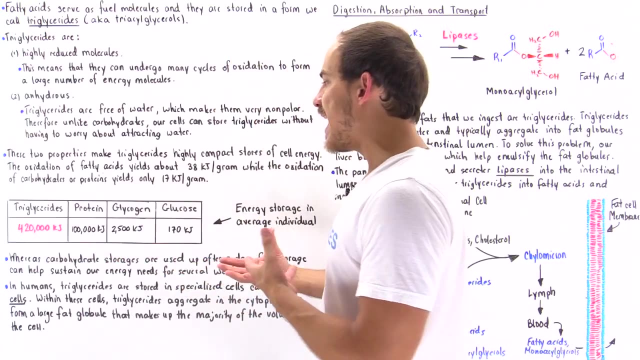 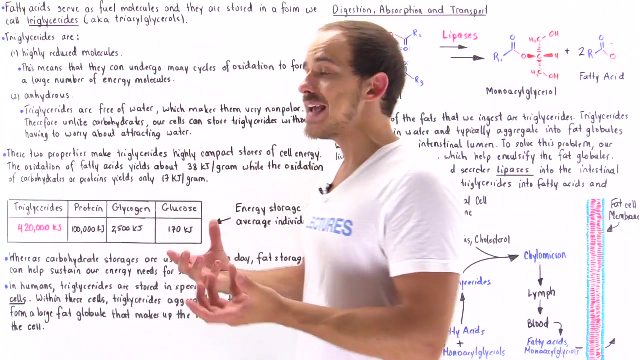 it makes up the predominant portion of the total energy that is readily available to the cells of our body. So we have 420,000 kilojoules of energy that is stored in triglycerides. So what that basically means is when we run out of these two storages of energy, our body will begin to break down the triglycerides to form the high energy ATP molecules, and that will last us several weeks And after we run out of our 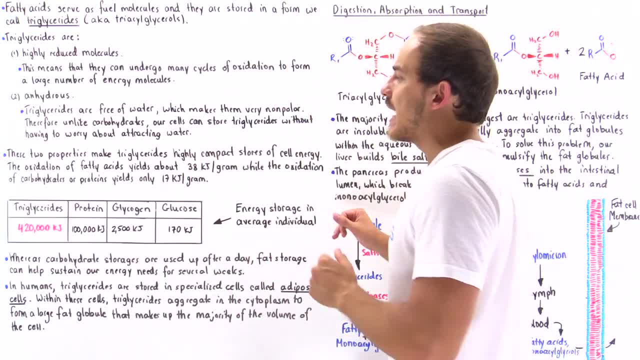 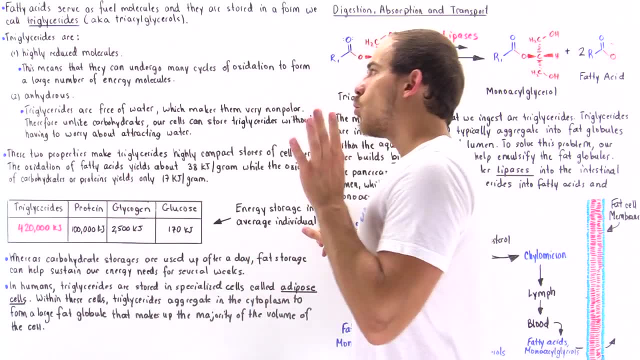 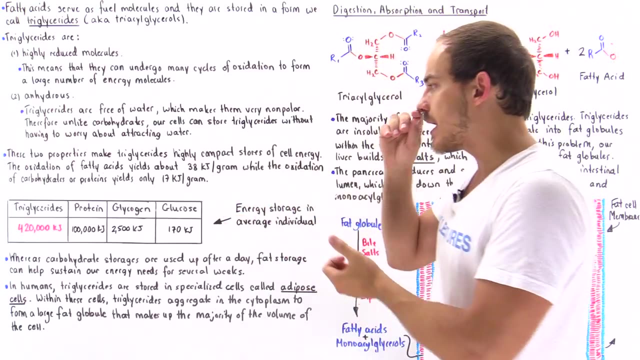 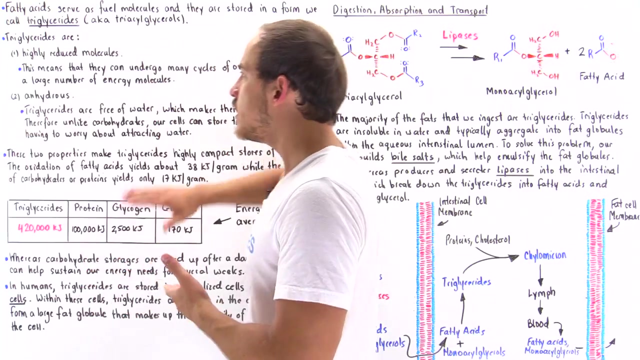 triglyceride storages. that's when our body begins to actually break down the protein, the muscles of our body for energy. Now the question is: what makes triglycerides so special? Why is it that our cells actually choose to store the predominant amount of energy within our fat molecules, the triglycerides, and not within, for instance, the glycogen? Well, these two properties make glyceraldehyde such a highly 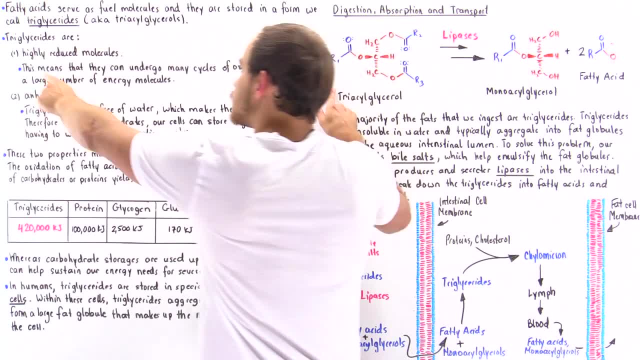 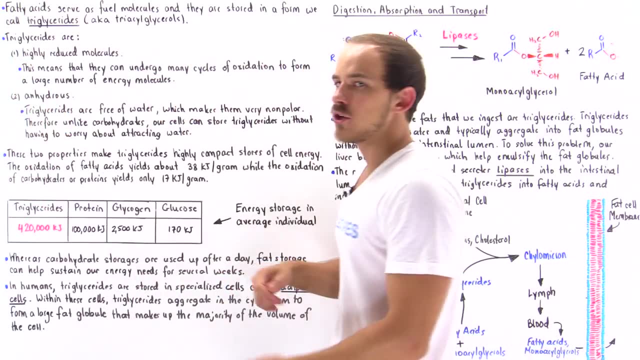 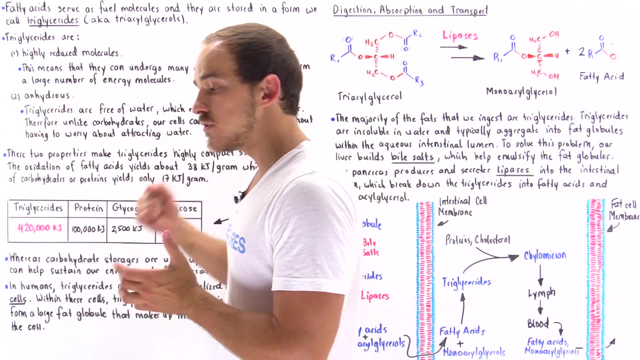 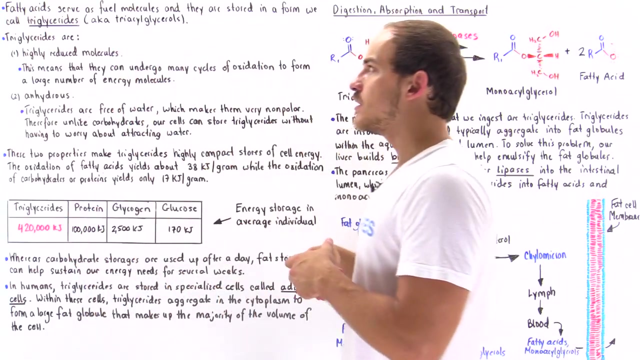 concentrated storage of energy. So number one is they're highly reduced molecules and number two is they're anhydrous. Now, what do we mean by highly reduced? Well, essentially, we have removed lots of electrons from the triglycerides. We have removed lots of electrons from the fatty acids, And that's important because we can actually break down the triglycerides via oxidation many, many, many times to produce a large number of 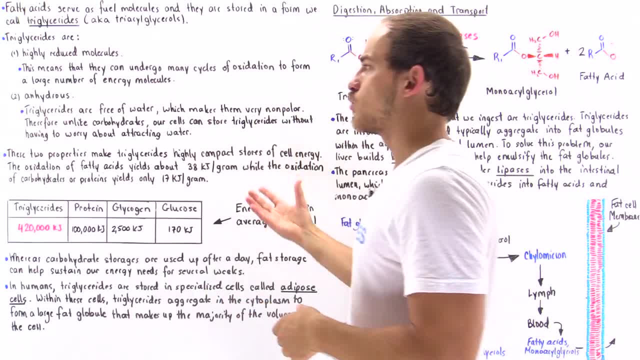 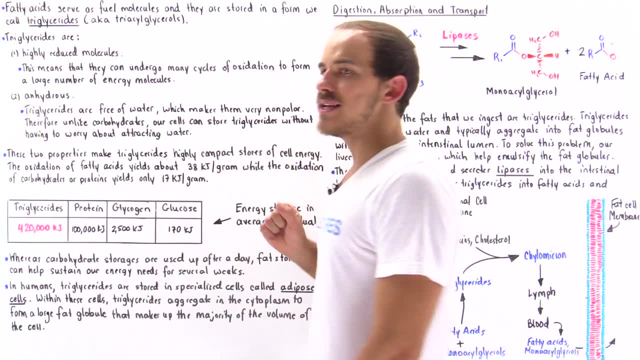 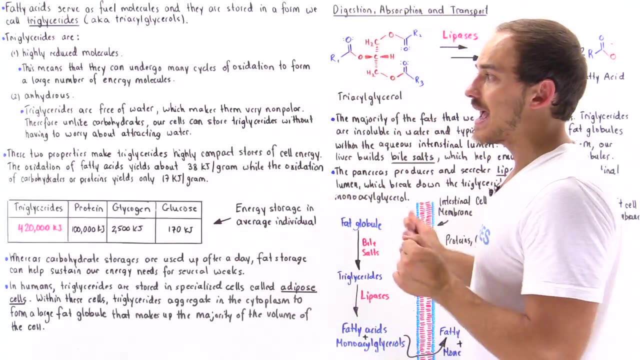 molecules that we can then use to help generate those ATP energy molecules. The second reason is the fact that it's anhydrous, And what that basically means is it is free of water. We don't have hydroxyl groups attached onto the fatty acids like we do, for instance. 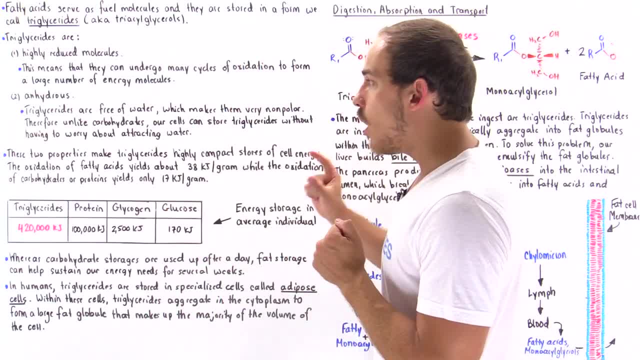 in glycogen, And what that means is water molecules will not tend to associate with fatty acid chains��, and what that means is the fatty acids, the part of the fat. use of hyaluronic acid free courses will not have the amount of law right and that is why we call those pigments as fat acid cancer and what we call those fat acid cancersuct. موج�ي counsel ces. 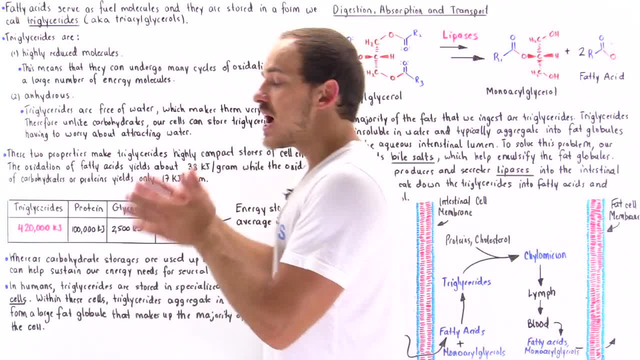 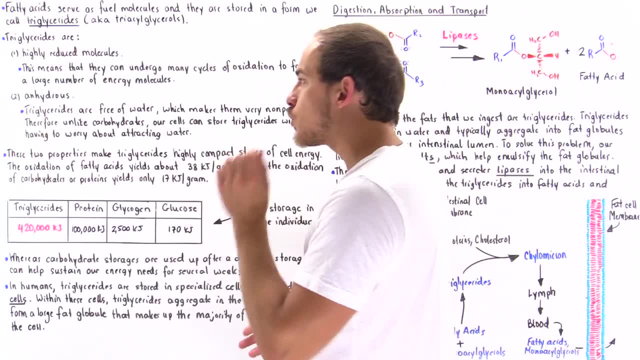 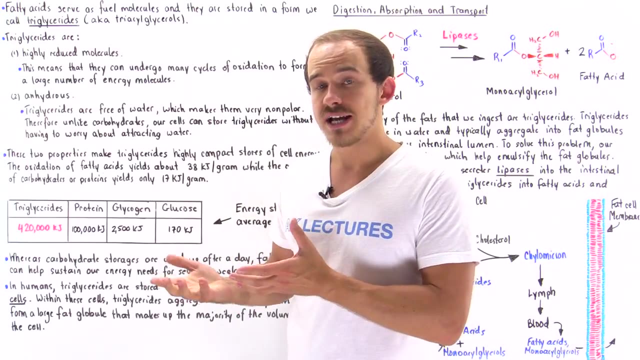 blanks actions. acids will be a much high, much more concentrated form of energy storage than glycogen. In fact, for one gram of glycogen, there are about two grams of water that associates with that gram of glycogen. Why? Well, because glycogen, which consists of glucose monomers, contains 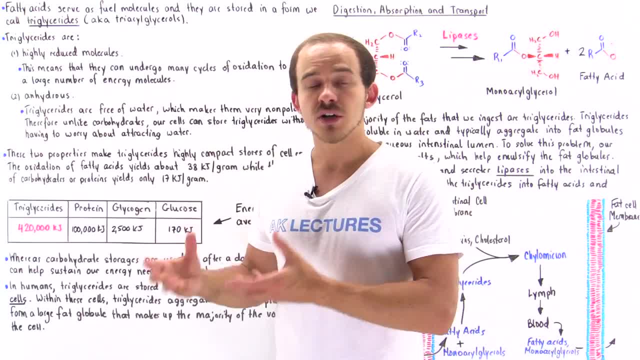 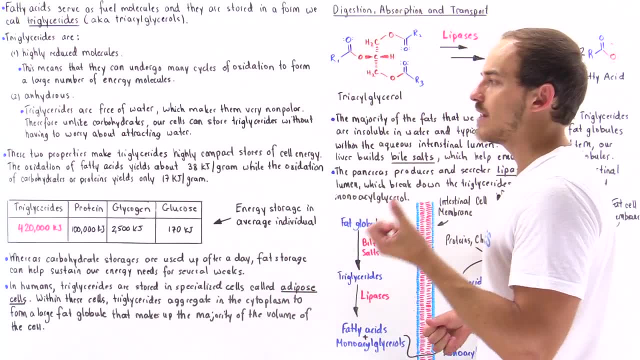 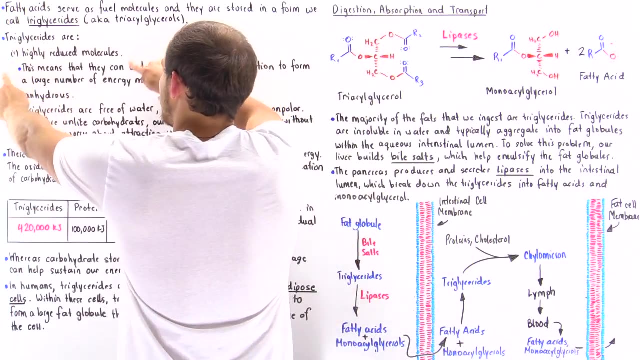 many hydroxyl groups, and those hydroxyl groups are polar and so they attract water, And so what that means is glycogen is not a very concentrated form of energy storage like triglycerides are. So we see that the fact that triglycerides are highly reduced and anhydrous, this makes triglycerides, highly compact and highly concentrated stores of metabolic cell energy. So the complete oxidation of fatty acids yields about 38 kilojoules of gram that we oxidize. And if we compare that to oxygen When we're oxidizing carbohydrates or proteins, this only yields about 17 kilojoules per gram. 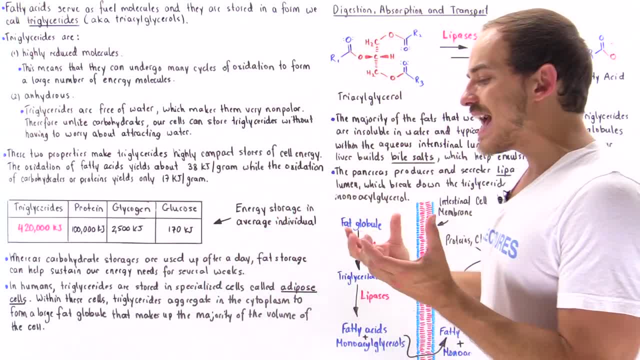 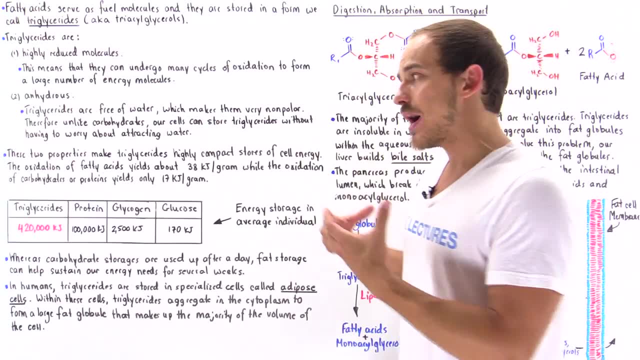 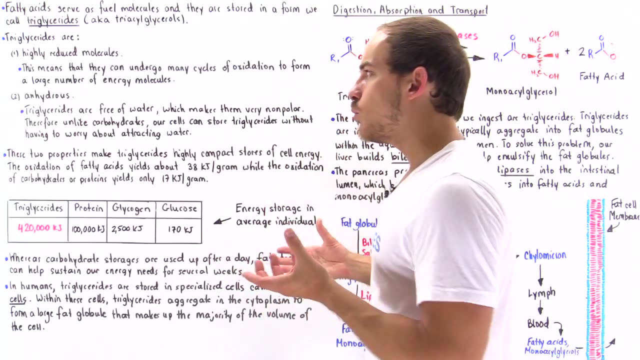 that we actually oxidize, So we're able to actually store much more energy in these fatty acids, And when we break down these triglycerides we can also actually form many more high energy ATP molecules. Now within our body we have different types of cells that can actually 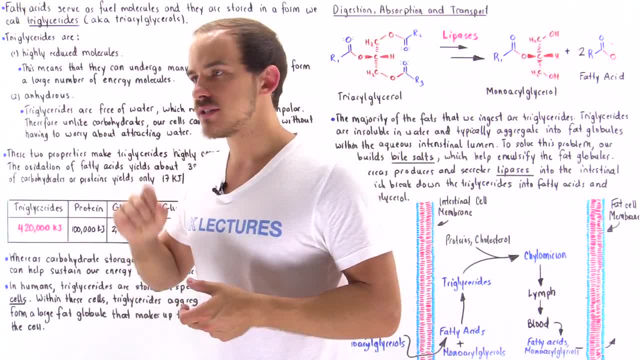 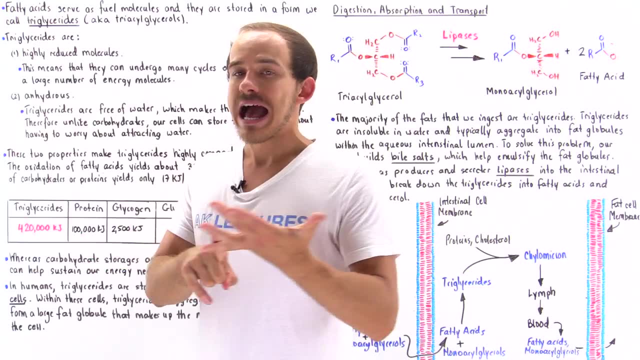 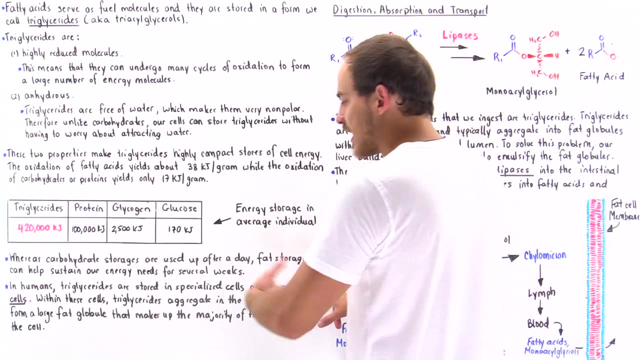 store fatty acids, But there are two most important cells, because these are the cells that store the predominant number of fat molecules, And this includes our fat cells, also known as adipose cells, as well as muscle cells. Now, these adipose cells, fat cells, are specialized in a sense that they store most of these triglycerides. 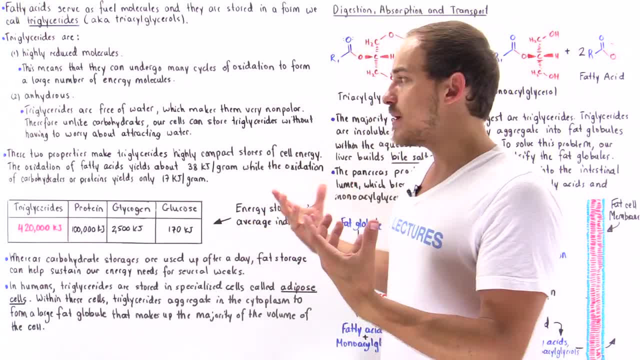 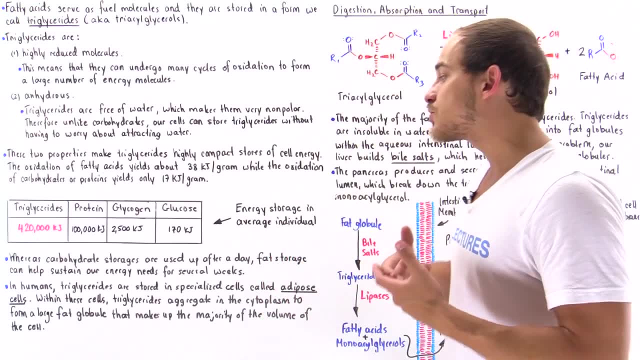 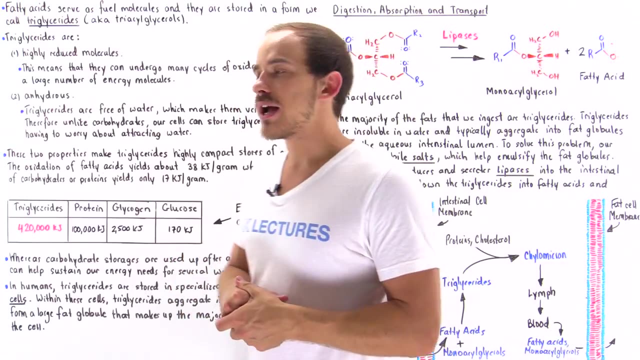 within their cytoplasm And these triglycerides basically aggregate together to form these large fat globules, And these fat globules actually make up the majority of the volume of these fat cells. Now, muscle cells can also store these triglycerides, And muscle cells store these triglycerides. 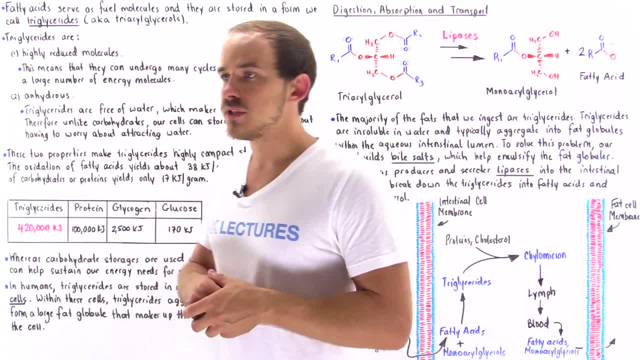 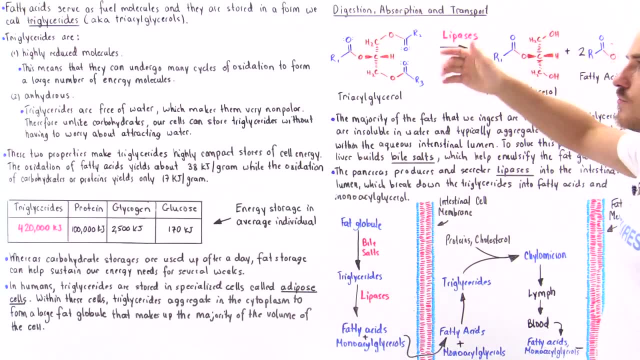 predominantly to actually use them for energy production, for ATP production. Now let's briefly discuss digestion, absorption and transport of triglycerides. So the majority of the fats that we actually ingest into our body in our diet are actually fat, And that's. 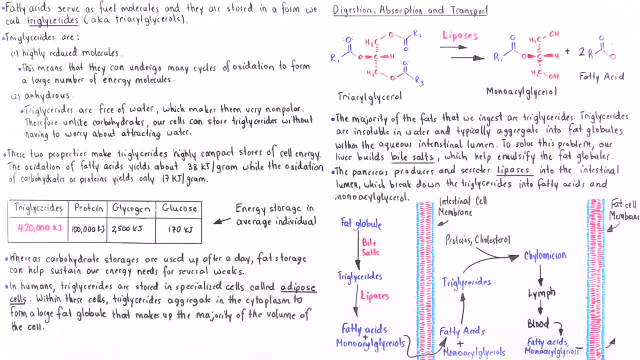 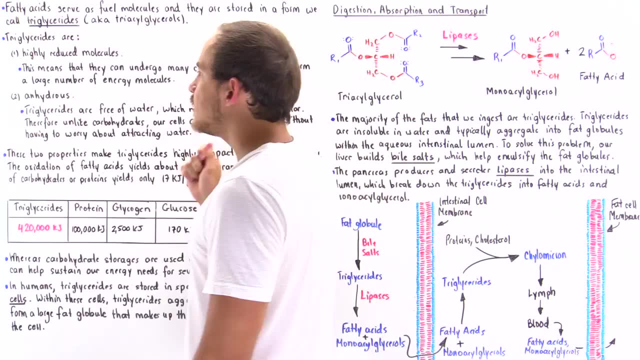 a very important factor. So what are the main factors that we ingest into our body in our diet? Basically, are these triglycerides. Now, triglycerides are, as we said earlier, are insoluble in water because they're non-polar. 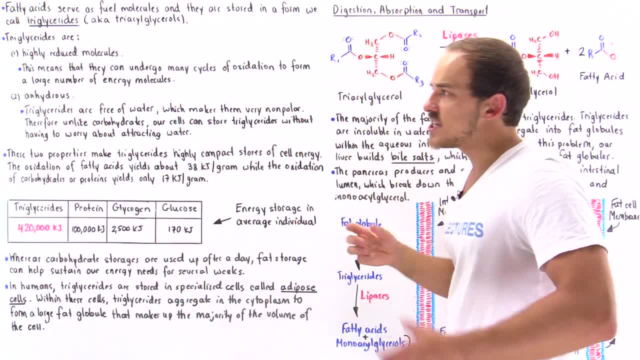 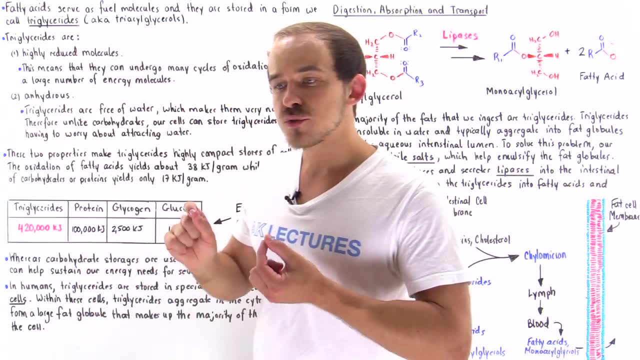 Remember, they're anhydrous And what that basically means is when we ingest these triglycerides into our body, when the triglycerides make their way into the lumen of our small intestine, because the lumen is an aqueous environment. it consists of water. 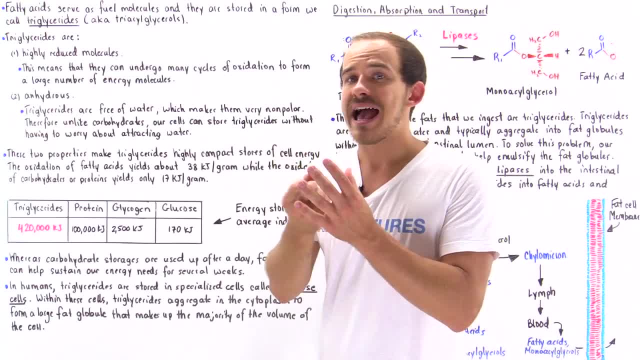 What that means is these triglycerides are insoluble in water. And what that means is these triglycerides are insoluble in water. So those triglycerides are insoluble because they're non-polar- werden Englisch. So when we ingest triglycerides, triglycerides are insoluble. they're insoluble in water. 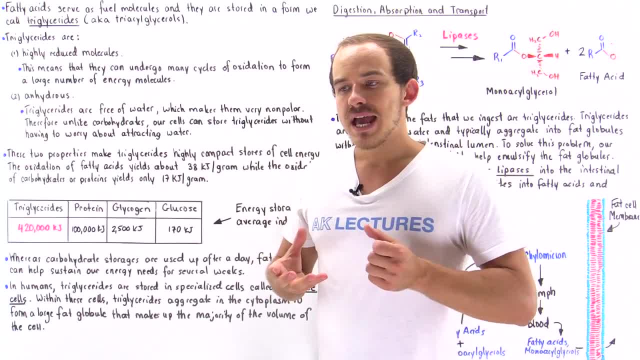 And what that means. what that means is we ingest them into our body. So what does triglycerides do? It's said that triglyceride can update our immunity system and help Winning overweight and Civicie. Your pancreas secretes special enzymes, proteolytic enzymes, known as lipases. 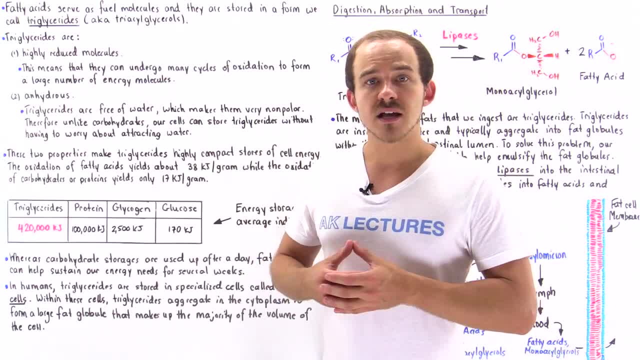 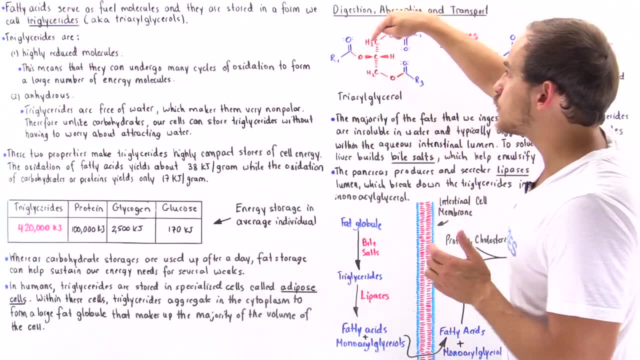 And these lipases are actually responsible for cleaving these ester bonds that exist within triacylglycerol. Now our pancreas secretes special enzymes- proteolytic enzymes- known as lipases, And these lipases are actually responsible for cleaving these ester bonds that exist. 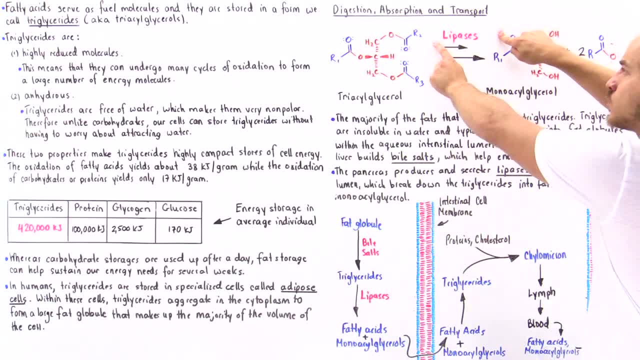 within triacylglycerol, acylglycerol. So we have lipases which can act on these bonds and when they cleave, let's say this bond and this bond, we basically form this mon acylglycerol and two fatty acids And once we 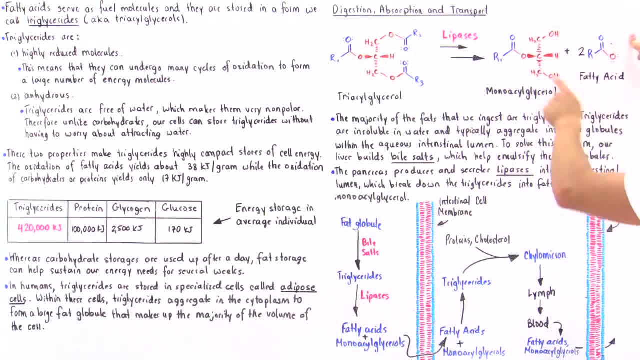 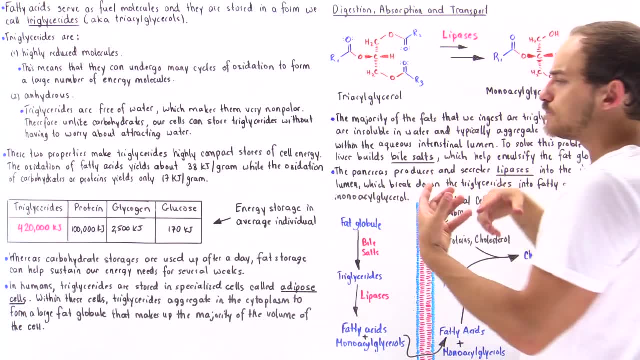 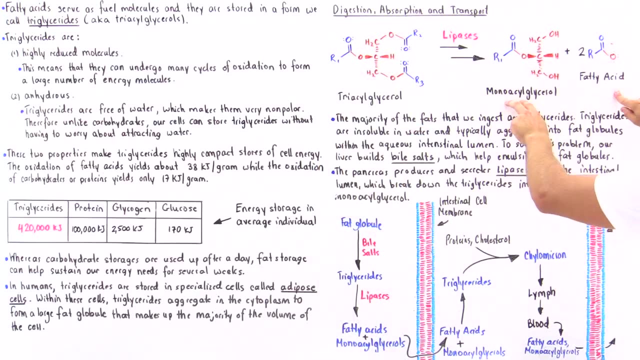 form these molecules. only then can these molecules actually be absorbed by the cells found in our small intestine. So our small intestine doesn't actually- or the cells of the small intestine doesn't actually- absorb the triacylglycerols. Instead, it absorbs these types of molecules. 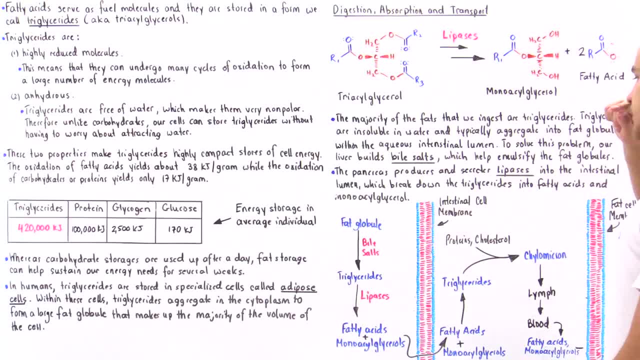 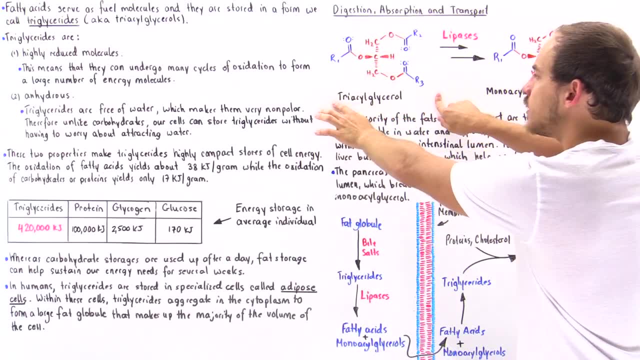 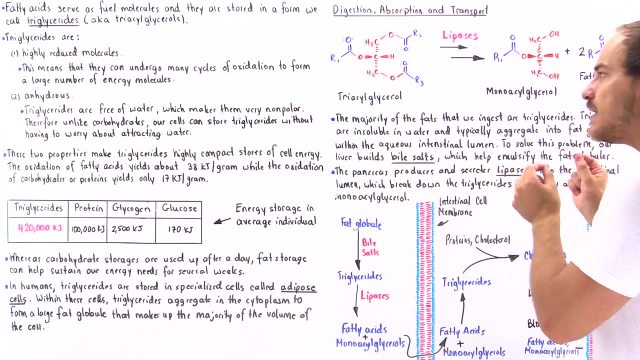 the constituents, the fatty acids and the mon acylglycerol. Now the problem is because of the fact that this is a nonpolar molecule and our lumen is predominantly an aqueous environment. we form these large fat globules and the lipase enzymes can't actually get to the majority of 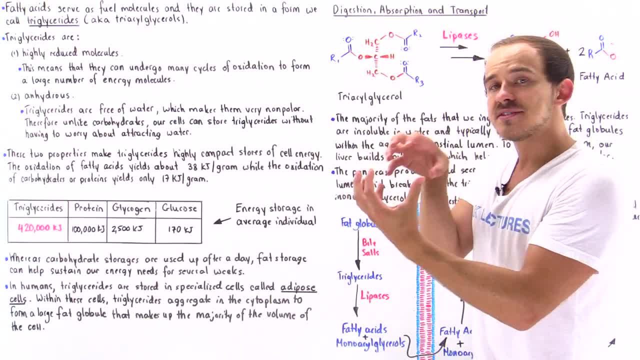 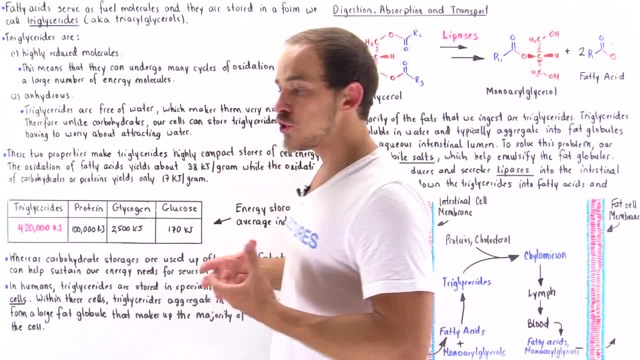 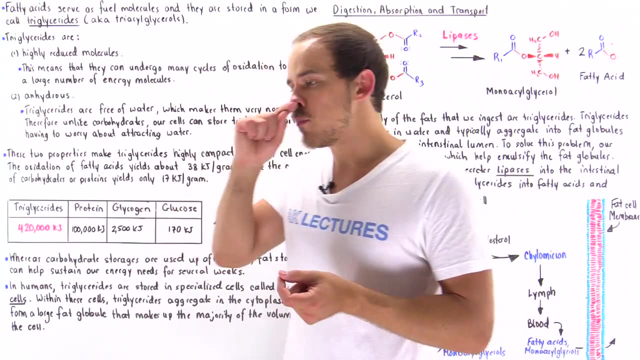 these triglycerides because they exists at the center of the fat globules, And so our liver basically uses cholesterol molecules to help build bile salts, and the bile salts are actually stored in our gallbladder and released into the small intestine. and once the bile salts, 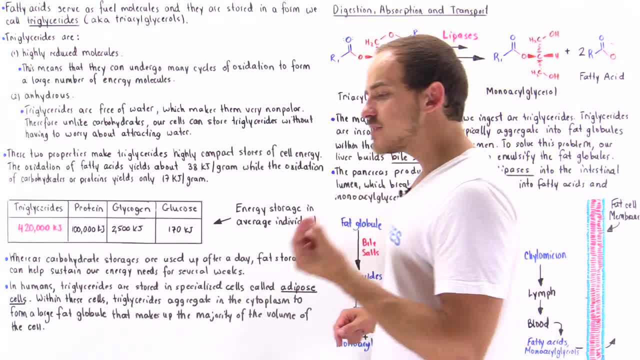 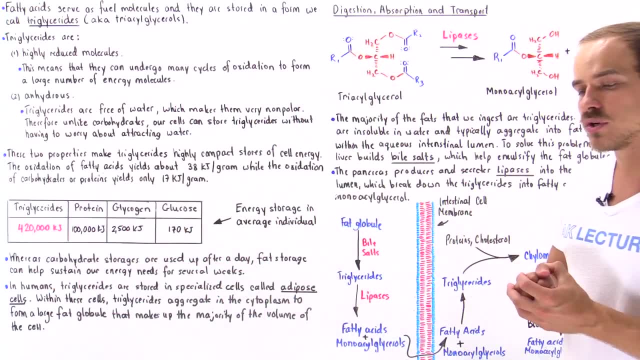 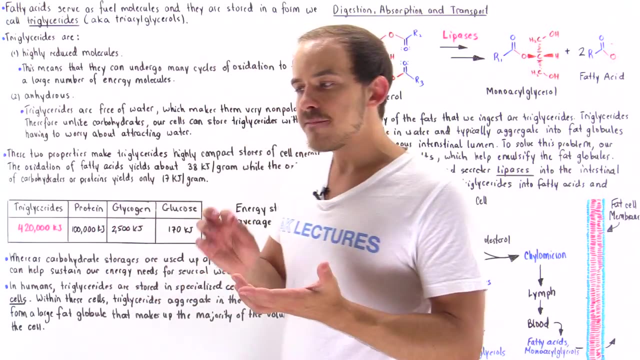 actually make their way to the small intestine. what the bile salts do is they begin to emulsify and break down those fat globules into smaller constituents. And what these, what these bile salts are, are? they're essentially these amphipathic molecules that can associate 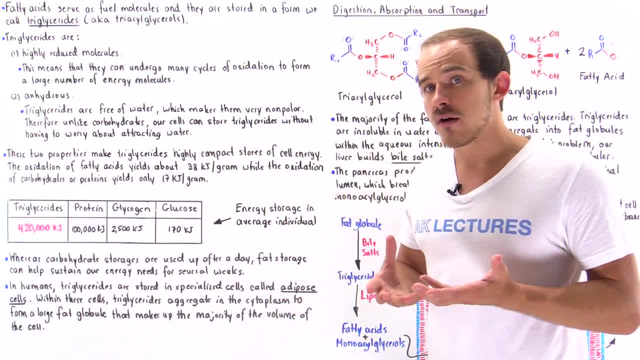 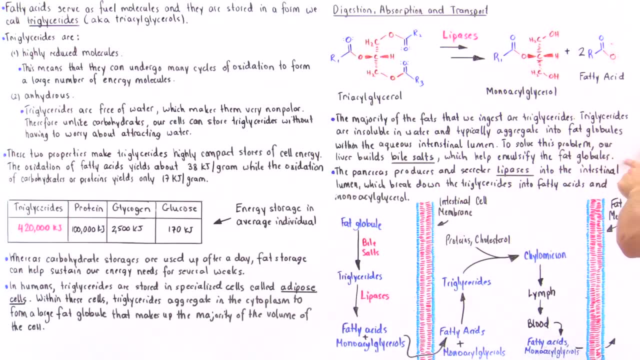 not only with the aqueous environment, in the lumen of the small intestine, but also with these fat globules. And that's exactly what allows them to actually emulsify and break down these fat globules. And once it breaks them down to the fat globules, then the lipases can actually begin. 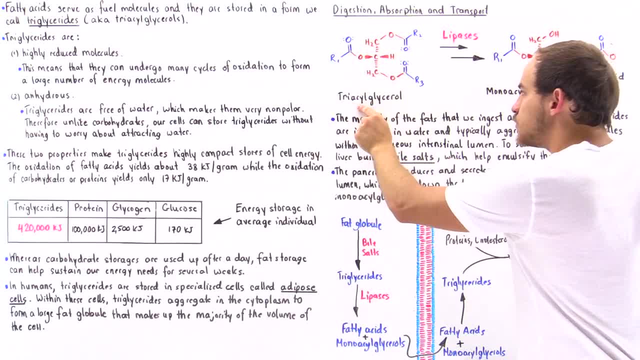 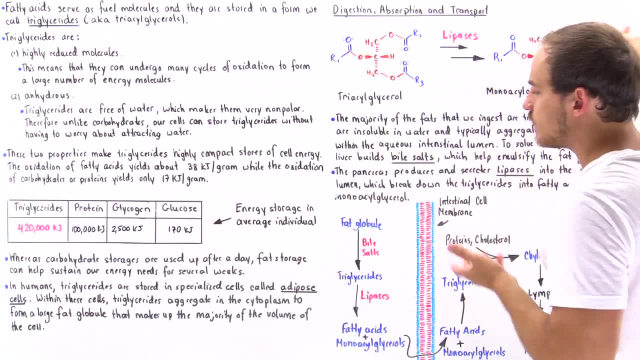 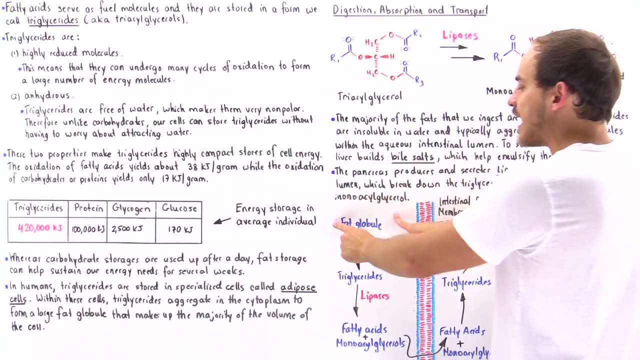 to act on the individual triacylglycerols and that can break them down to these two constituents, which then can be absorbed by the cells found in the lumen of our small intestine. So in the lumen we basically have these aggregates of triacylglycerols, the fat globules. 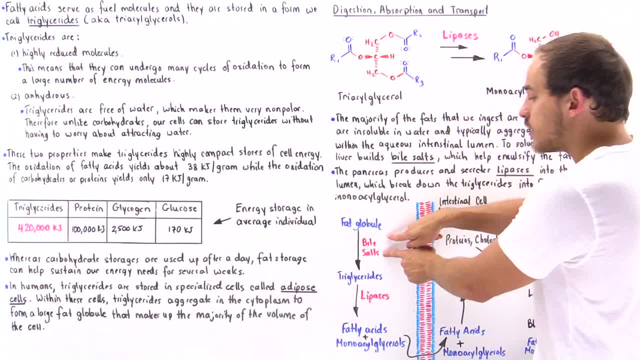 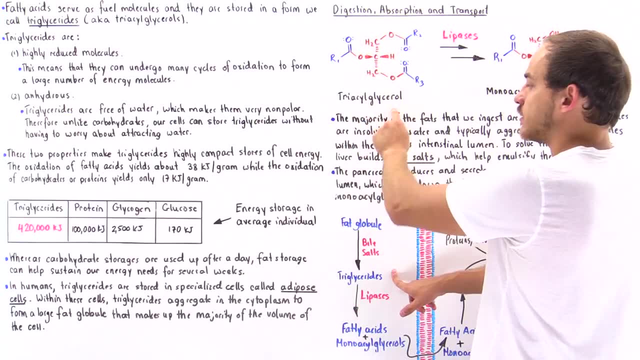 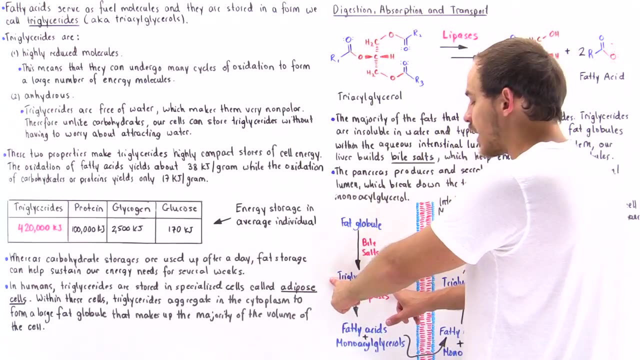 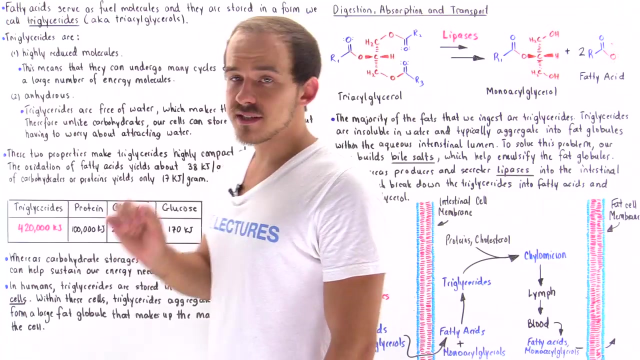 when our gallbladder basically secretes the bile salts, that helps emulsify them into triglycerides or triacylglycerols, And then the triglycerides, or the lipases, act on these triglycerides, breaks them down into fatty acids and monacylglycerols, and then those are absorbed by the cells found in the small intestine. 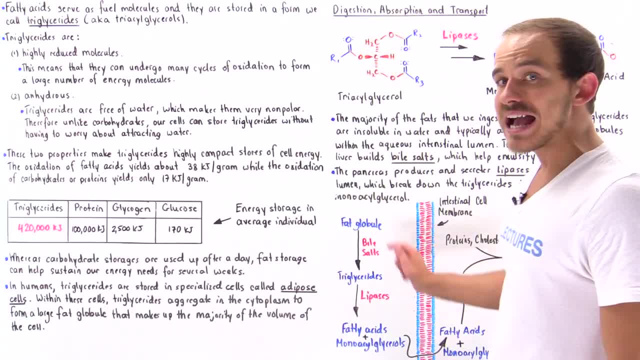 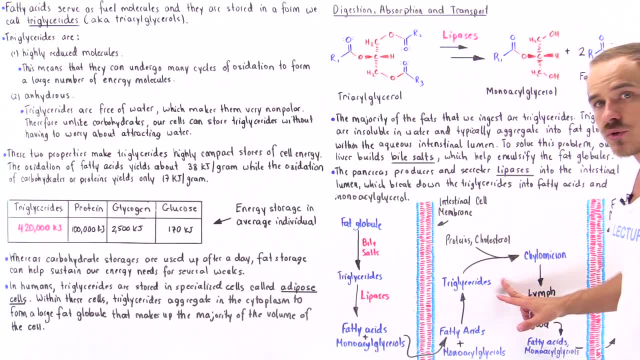 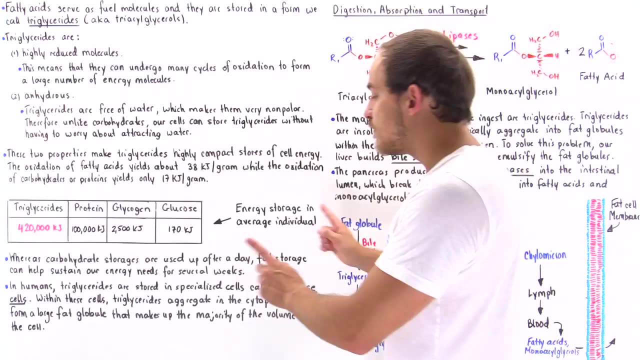 And once these fatty acids and monacylglycerols actually make their way to the cell, into the cytoplasm, they are then used to resynthesize the triglycerides. Why? Well, because these actually need to make their way to the target cells: the fat cells and the muscle cells. 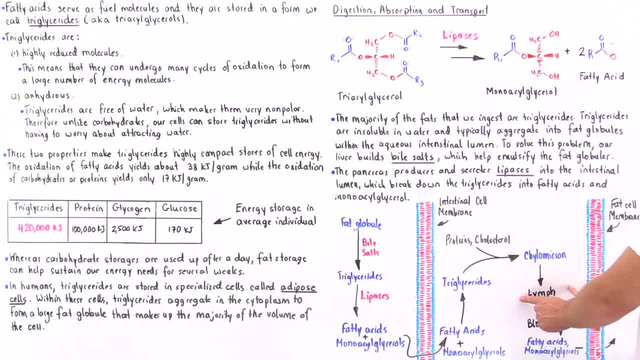 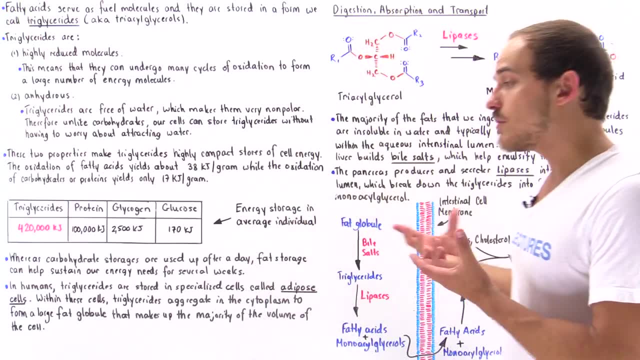 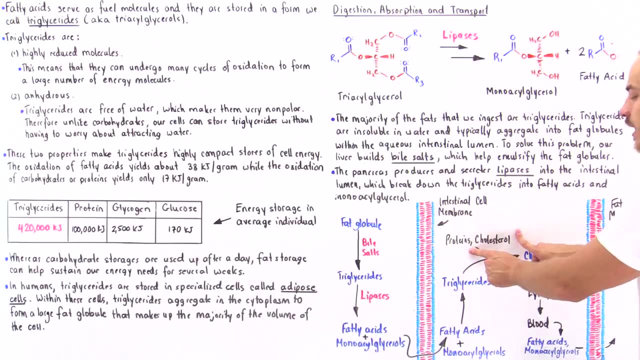 And so triglycerides. before actually making their way into the lymph system of our body, they are placed into these carrier molecules, carrier particles known as chylomicrons. Now, a chylomicron basically consists of proteins, cholesterol molecules, phospholipid molecules. 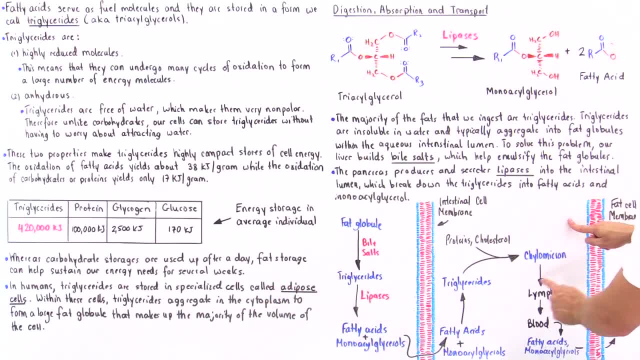 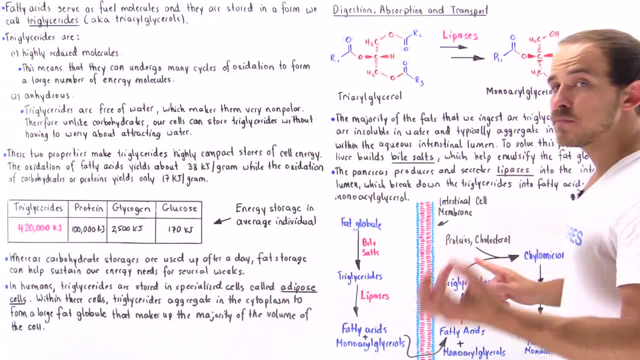 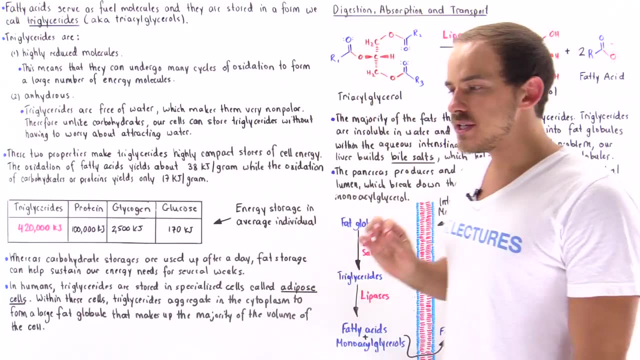 fat soluble vitamins and other molecules, but the predominant portion of these chylomicrons are triglycerides. In fact, triglycerides make up about 90% of the portion of the chylomicron. Now, once we form these chylomicrons, they then move into the lymph system and then they 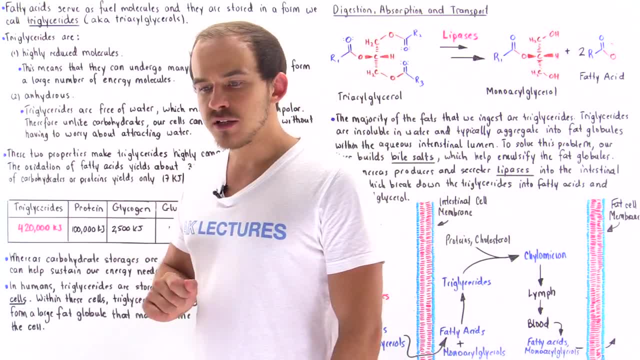 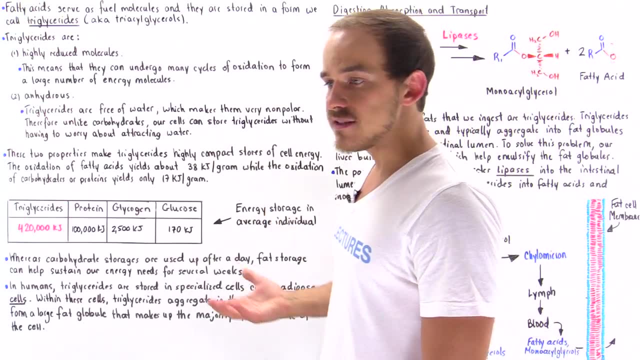 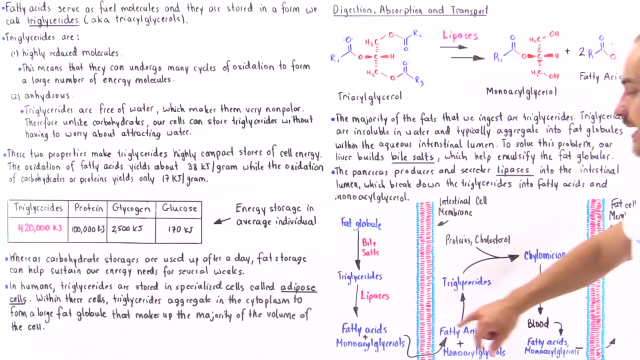 travel into the blood plasma And once inside the blood plasma, these chylomicrons move onto the membranes of target cells, So cells like adipose cells, fat cells or muscle cells- And once they attach onto the membrane, they once again are broken down back into the fatty 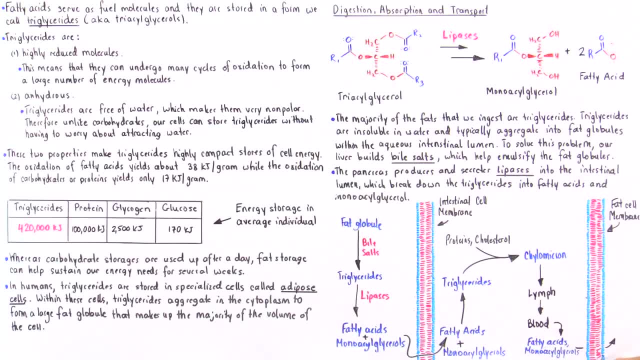 acids and monoacylglycerols, and then those are absorbed by that particular cell. And so, if we're talking about fat cells, once these are ingested into the cell they are then converted back into triglycerides and then those triglycerides begin to basically 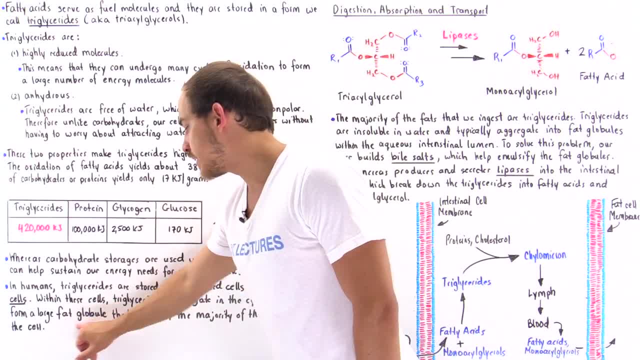 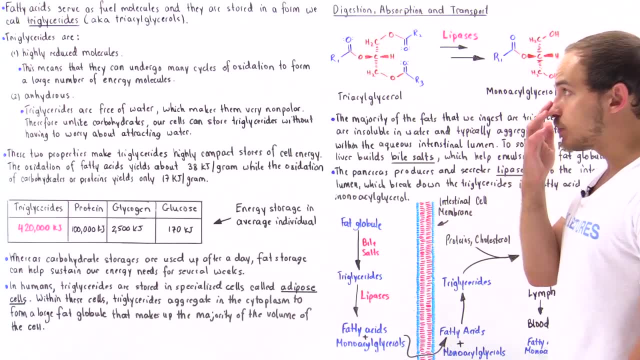 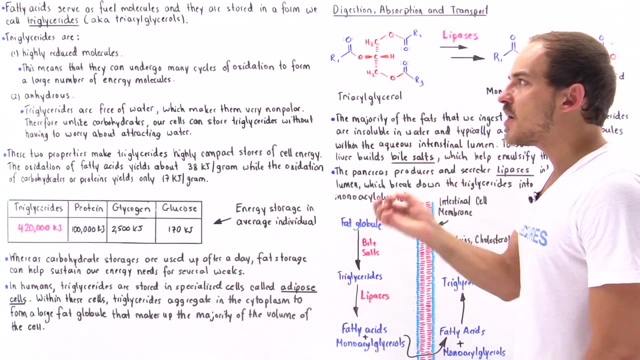 aggregate together. Okay, And that's how we form these large aggregate molecules known as fat globules. So we see that the takeaway lesson from this particular lecture is the fact that these triglycerides are very, very specialized, in the sense that they're very highly concentrated. 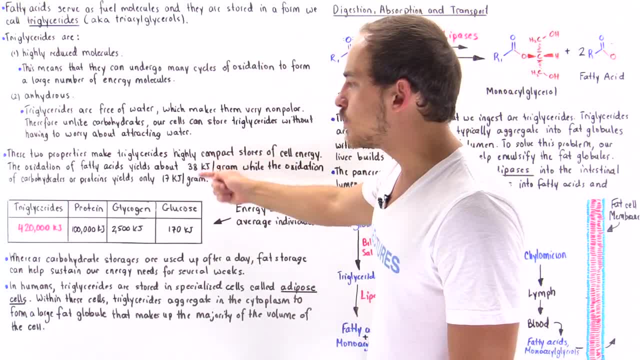 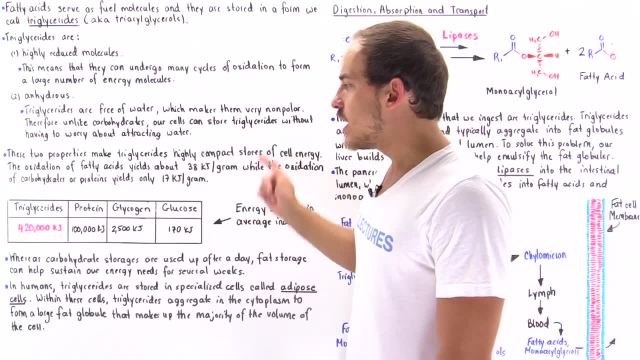 forms of energy storage. Compared to glycogen and protein, we're able to actually store much more potential energy within the fat molecule, the triglycerides, than the proteins. Researchers are able to Just forget the non. You're still listening on a radio show. You're listening to an audio show. We'll see you next time. Have a good one And stay connected, Thank you. 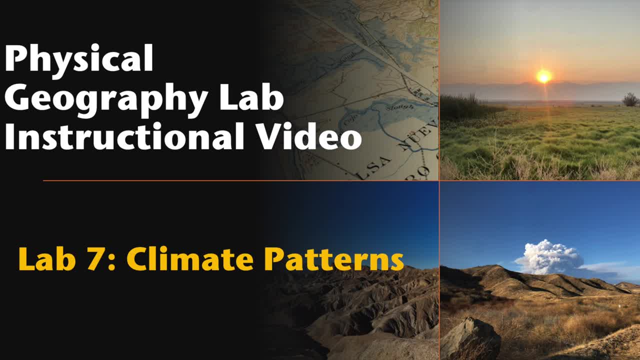 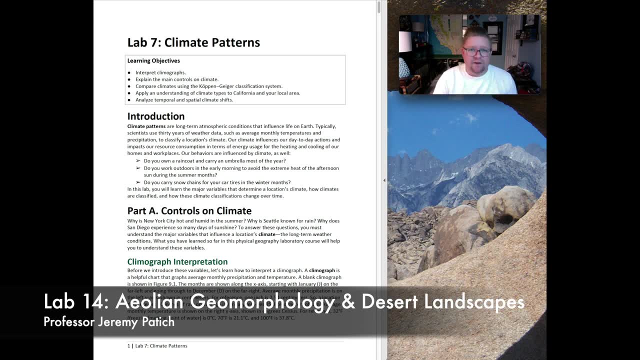 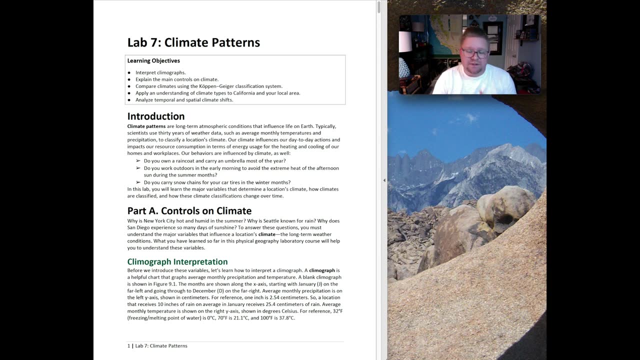 Hello and welcome to Lab 7, Climate Patterns. This video is being provided for you so you can see and have the instructions by page by page, step by step, where I'll provide some hints, tips and some tricks to work through this lab efficiently and effectively. 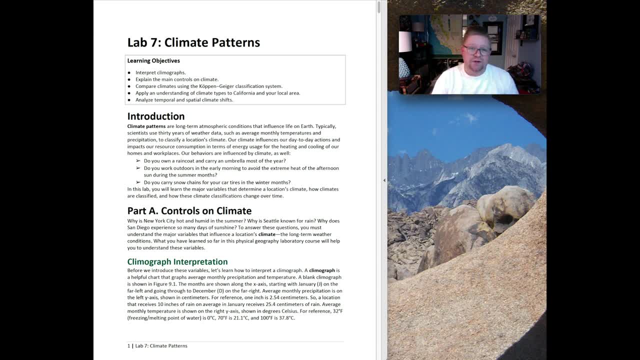 This is also going to be helpful, especially as you are working through your course, whether it be face-to-face or online, so you can reference back and see an explanation on how some of the math and concepts are completed. I find them very helpful when you're reviewing for exams, because perhaps you forgot how to do a certain part or you weren't sure what that meant. You're able to come back to these and check out the chapters that have been separated within this lab to see it. 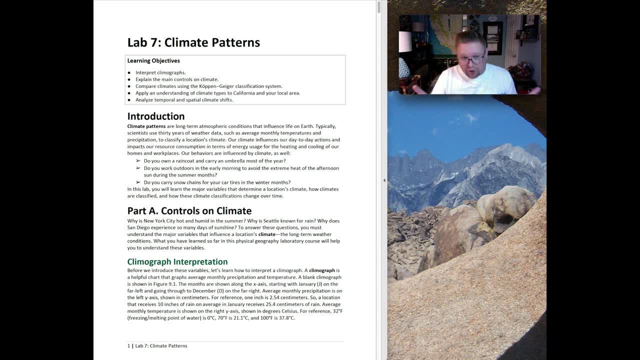 Now we can see. the learning objectives for this lab are to learn how to interpret climate graphs. To explain the main controls of climate, compare climates by using the Köppen-Geiger classification system. to apply an understanding of climate types in California and your local area. and to analyze temporal and spatial climate shifts. 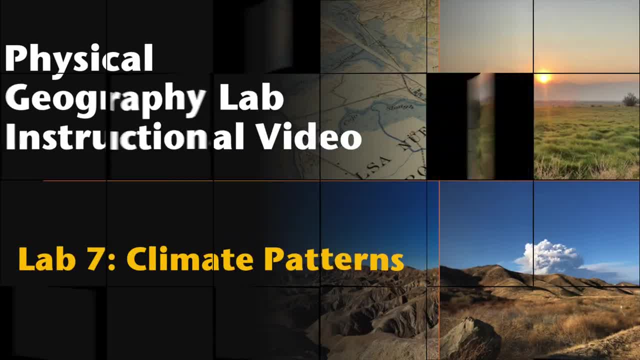 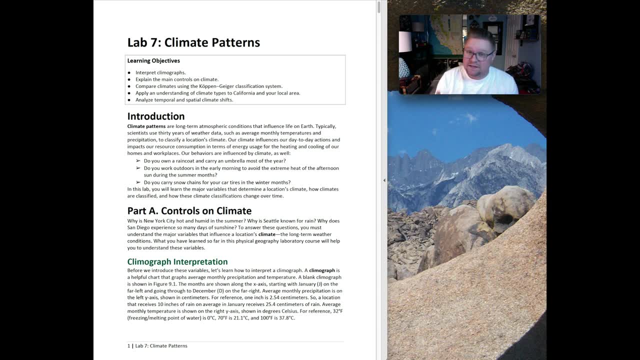 That being said, let's start Lab 7.. So climate is obviously a catch term that's being very popularized right now. You know, I think let's start with climate. Let's start with climate. What's important to understand about climate is that climate is a lot different than just weather.